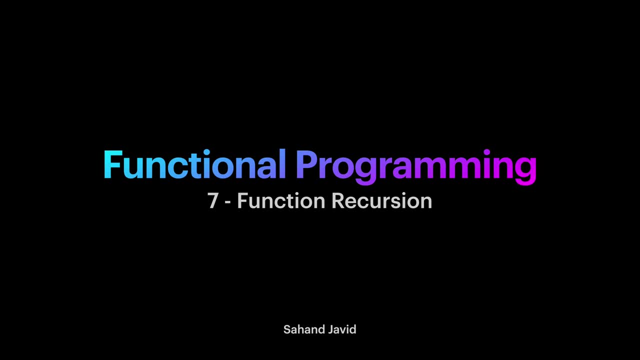 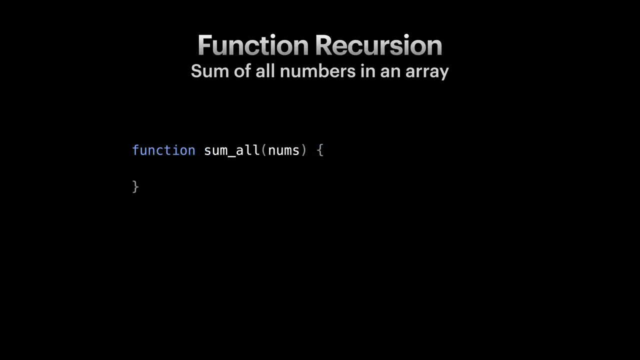 In the previous videos I mentioned, there are no for or while loops in functional programming. In this video, we will learn how to model loops in functional programming. Let's look at this by an example. We want to define a function, sumAll, which receives an array of numbers and return the summation of those numbers. 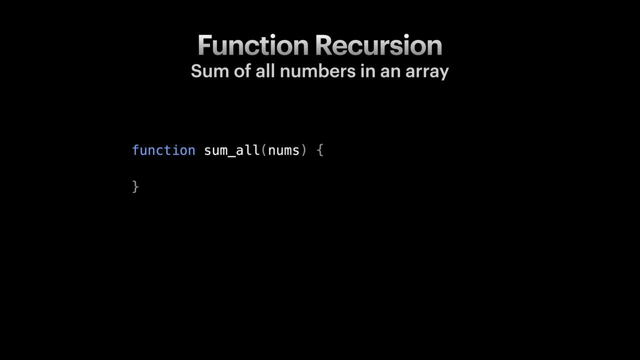 In an imperative approach, we would come up with something like this: We define a variable for keeping our result, initialize it with value 0, then iterate over the array items one by one and update the result by keep adding each number to it. 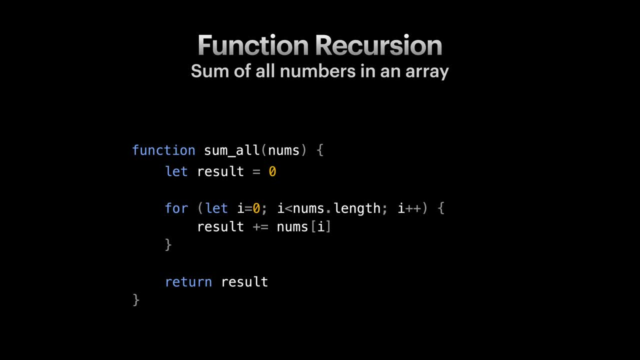 In other words, we keep mutating variable result until it gets to our desired state. As I mentioned before, we don't do mutations in functional programming. We believe mutation is dangerous and source of human errors and bugs. Then how can we model the sumAll in functional programming? 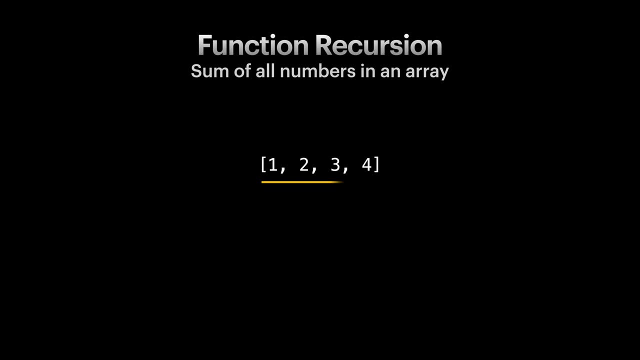 Let's take a closer look to our array. We want to return the summation of all the numbers in the array. Can we look at this in another way? Let's split the array in two parts: The first element of the array and the rest of the array. Wait a second If I've already knew the summation. 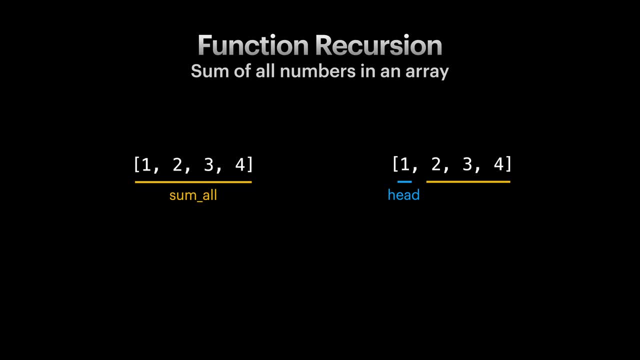 to the rest of the array by just adding the head to it. isn't it the answer to the whole array? That's the aha moment here. The sum of 1, 2,, 3, 4 is the same as sum of 2, 3,. 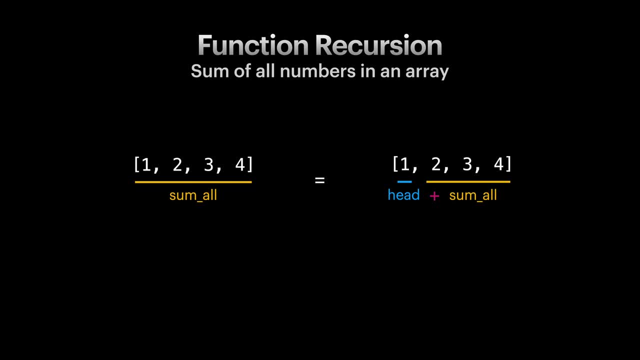 4 plus the head, and that is why it is called recursive, because we use the function to define itself. If this is a bit mind-bending, pause the video and think about this. If you understand this part, then you've understood recursion. There is one thing left: What if?